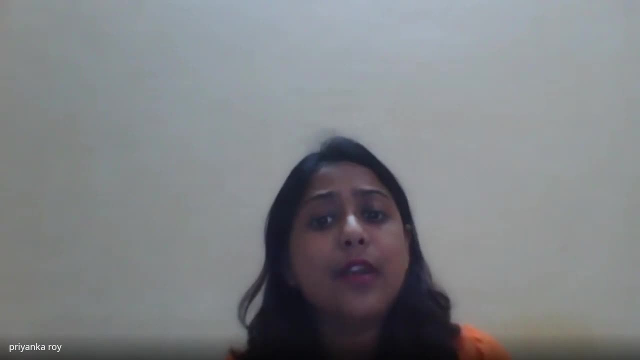 drought-like situation, Then we will try to identify and understand what are the areas, that is, the zonation of drought. okay, So what are the areas which is, you know, completely prone to drought and why it is prone to drought-like situations? Why not all parts of the country is not, you know, falling prey to a drought, but only a few. 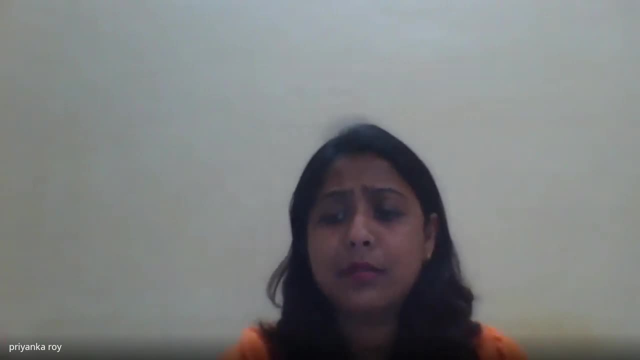 regions in the country. Why You know there are. there is an interior part of the country which is very prone to drought. There are also seen that there are areas and places which are receiving heavy rainfall during monsoon season, during the raining season, but are, you know, still affected by a dry spell and resulting into, you know, low yielding of your agricultural products during that dry spell season, right? So at the end of this we will understand key: what are the causes of drought, what are the effect of drought and how we can manage and mitigate the effects of drought in the country. all right, 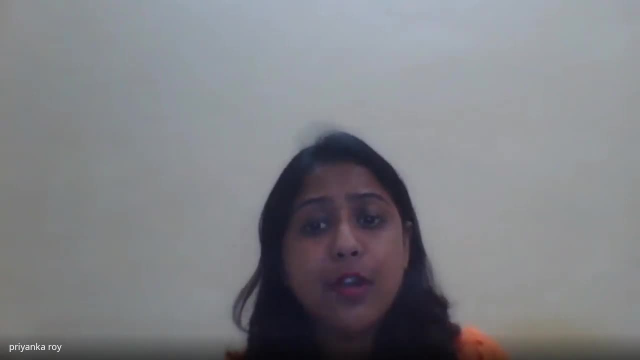 So we will also try to address the. you know the history and historical background and events that has happened in case of a drought, right? So coming to the, the point back is drought. drought is a is a process where you know the rainfall is. short, all right. The shortage of rainfall causes drought. okay, Now US Weather Bureau defines drought as a period of dry weather for sufficient length and severity to cause its at least least and partial crop failure. So least to partial crop failure is one of the signs that it is a drought year. 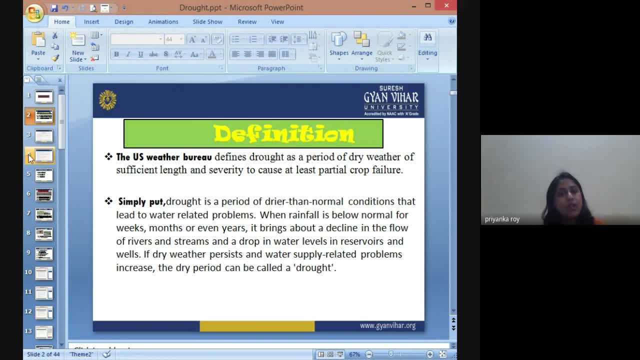 Simply putting, drought is a period of drier than the normal condition that leads to weather-related problems. So when rainfall is below normal for a week, month or even year, it brings about a decline in the flow of you know river. 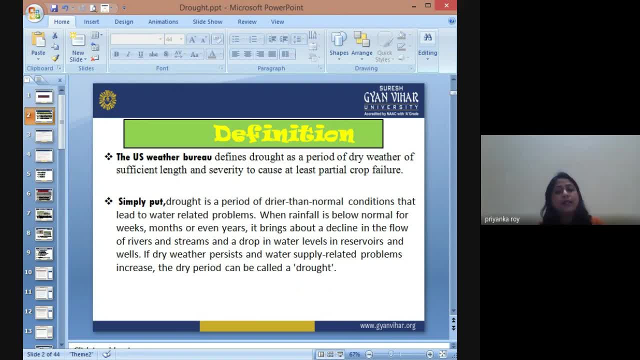 Water, then streams, then even other water bodies also decline in its water content. right, So water supply, when there is a shortage of water supply, problem increasing. that is a dry period, which is which we call is a drought year. okay, So drought is one of the world's most costliest natural disasters that happens. It is a slow onset of disaster, but it is one of the most expensive that affects the country, So causing an average of about $6 to $8 billion global damage annually because of the drought. And this has been done by the Kansas and UCAP in the year 2002, has studied and come to a conclusion that the drought is a catastrophic event which is causing about $6 to $8 billion loss every year Now, according to him. well, you know. 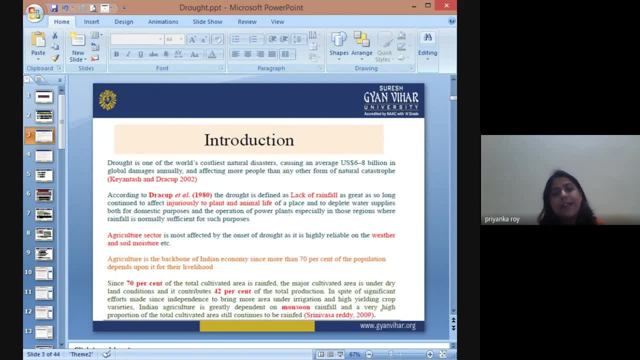 You have explained that the drought is defined as a lack of rainfall as great as long it continues to affect the- you know injurious affect the plant and injury the plants and animal health and well-being. Okay, So the place and where it depletes the water supply depletes both the domestic purpose. 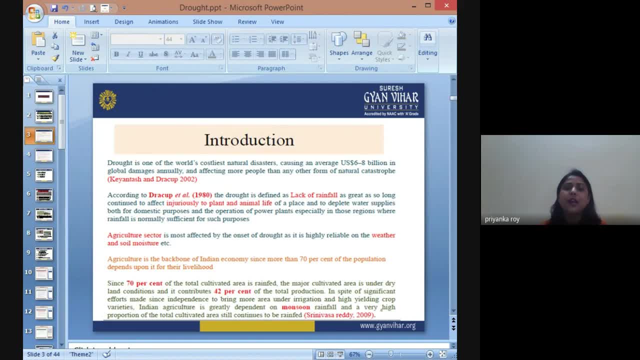 and the, you know, natural processes are affected by the drought. Okay So, agriculture is the sector which is mostly affected by a drought condition. Okay So, in any agriculture sector which is, you know, depend on obviously, all the agriculture, 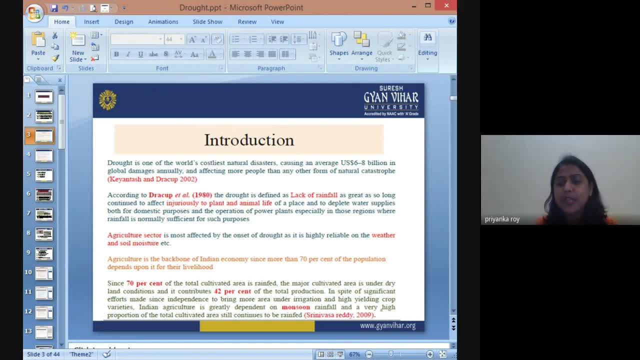 sectors are dependent on water. Okay, Irrigation. So if the regions of the areas do not have appropriate or sufficient amount of water for irrigating that field, what will happen is these plants that they have sown will not timely germinate, will not, you know, even if they grow, but they will not be able to. 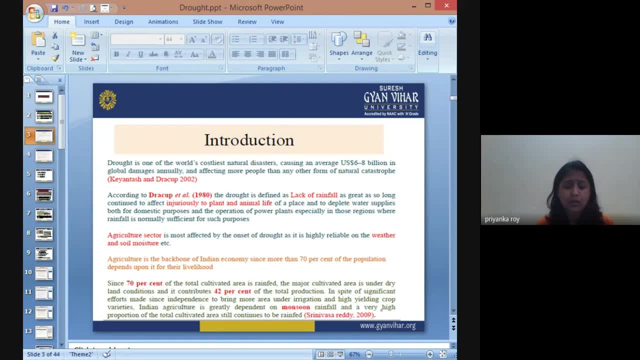 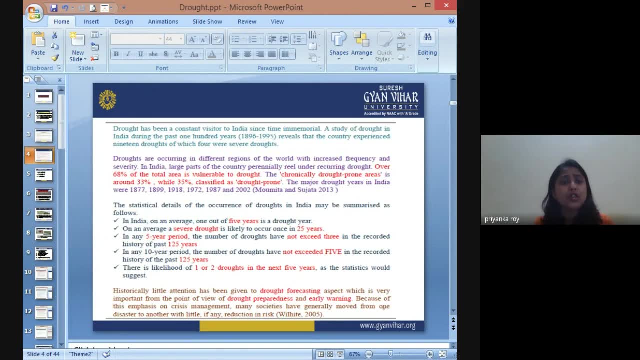 yield the proper. what do you call? you know the production, agriculture, production. the yield will not be as to the mark. So drought has been a constant visitor in the Indian continent. Okay, So in India it has been a constant phenomena. 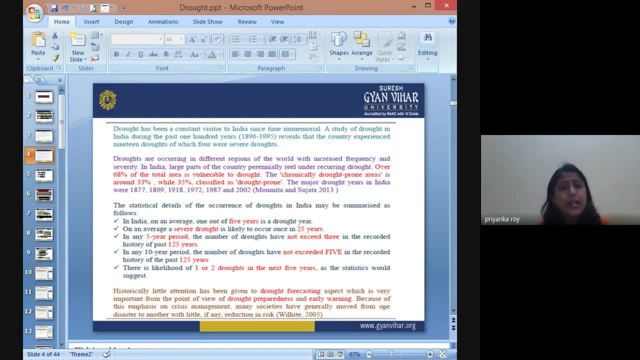 Okay, So a study of drought in India during the past one year. Okay, So a study of drought in India during the past one year. Okay, So a study of drought in India during the past one hundred years. that is taking from. 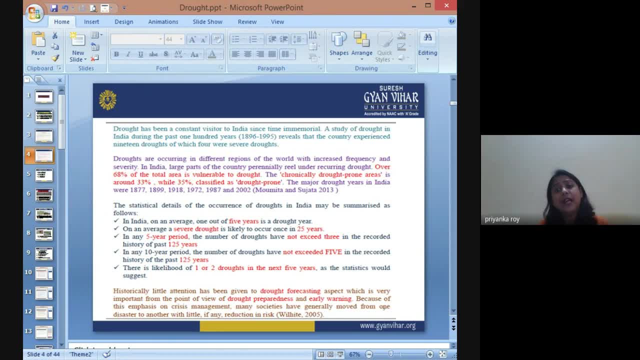 1896 to 1995 reveals that the country experienced 19 drought, of which is four were very severe. So four severe droughts were experienced by the country in past a century. Okay, So these past century that has seen a severe effect of dry spells. 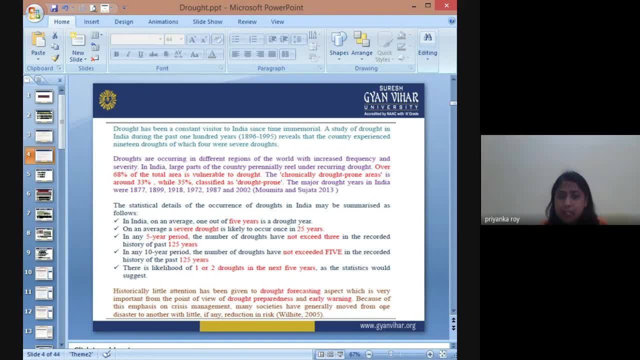 The drought occurring in different regions of the world with increased frequency. It is also I paid a very potential part in the Are our Indian subcontinent. in India, large part of country That is perineal, really real and under recurring drought, over 68% of the area is more prone. 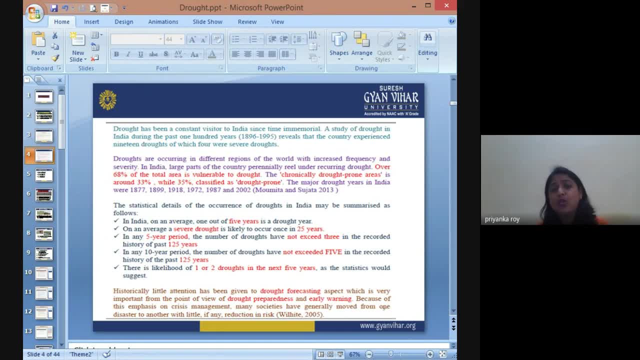 to drop. in our country is about 68% of the land which is prone to draw. the clinical drought prone areas is a what. What is the nailed up to the healthy? uh Yeah, about 33 percent, while 35 is classified as a drought prone areas, so chronically drought prone. 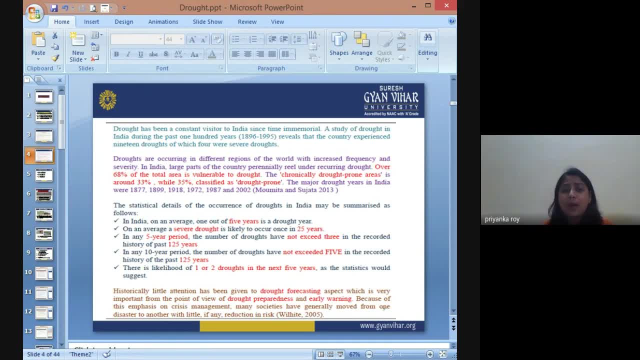 areas, that is, the severe drought prone areas, are about 33 percent and out of which, again out of 68 percent, there is 35 percent of the land which is prone to, you know, moderate to moderate drought. the major drought years in the country that were recorded are 1877, 1899, 1918, 1972. 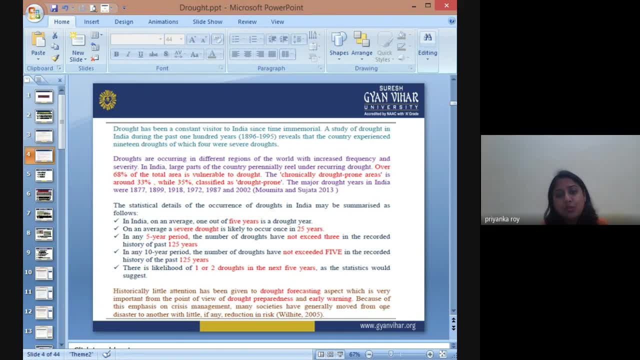 1987, 2002, uh has been recorded as a, you know, significantly drought year. so it this is has been taken from the study of maumita and sujata study in 2013. the statistical details of the 추천 century caught the ah studies of the uh. Cauca umbrage study showed a considering growth. 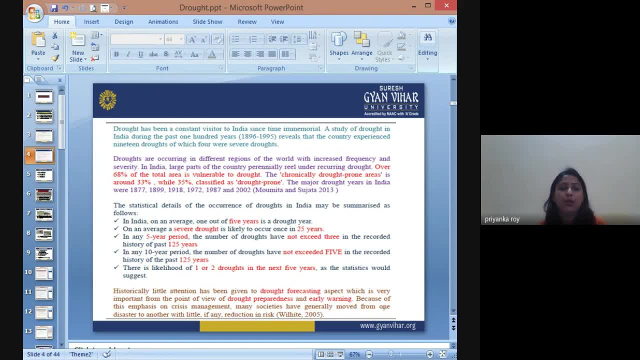 occurrence of the drought in India may be summarized as follows. like in India? uh, on an average, one of our five year is a drought year. uh, okay. so on an average, a severe drought is likely to occur in every 25 years. all right, so in five year period, the number of drought have not exceeded. more than three in the recorded history of 125 years. okay, so in last 10 year period, the number of drought have now exceeded more than five as compared to in the previous 125 years. so in recent times in past 10 years, what we see is that it has been seen, that we have been seeing. 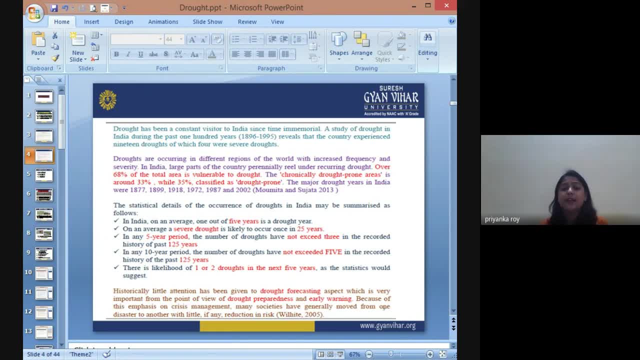 uh, the drought spell increasing, uh, you know, more than five times in a five year period. okay, so there is a likelihood of one to two, uh, droughts in every five years, as a statistic would suggest. all right, but now it. if you see, in the current scenario, if you go into 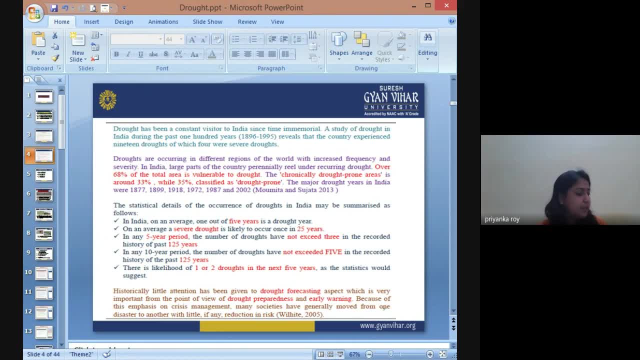 the field. there are many parts of the country wherein, during the summer season of the draw, dry spell faces a severe dry uh drought like situation where the agriculture product and agriculture field is dried up and does not yield anymore right. so historically little uh attention has been given to drought forecasting. 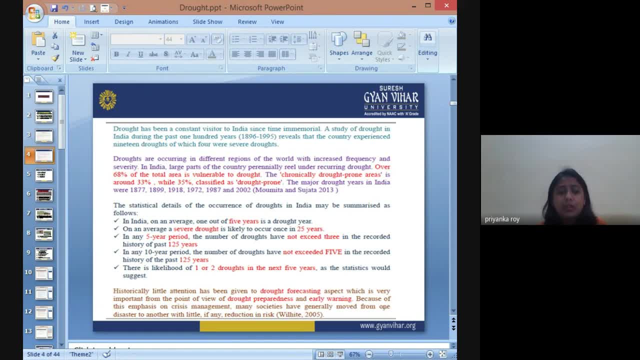 As aspects, which is, you know, very important for the point of view of a drought preparedness and early warning. because of the emphasis and the crisis management many societies have generated and moved one disaster into any other. little you know, it has moved into more active disaster rather than this one. 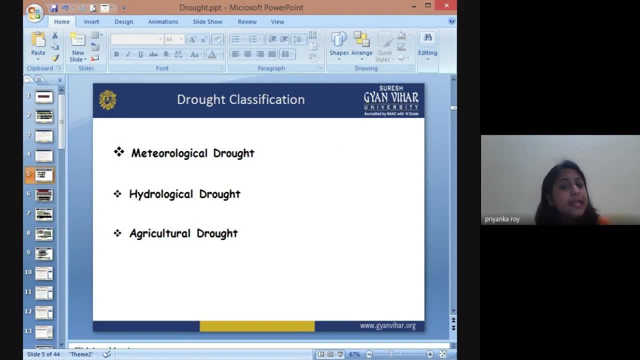 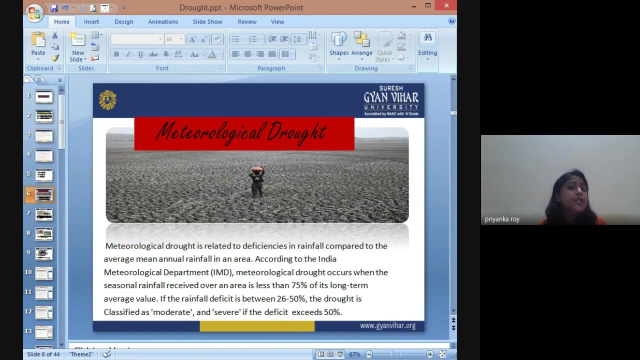 All right, But it has an effect on your daily life patterns. So metrological drought, hydrological drought and agricultural drought are one of those classifications of drought. So metrological drought- What is a metrological drought? A metrological drought is related to deficiency in rainfall compared to the average mean rainfall received in that area. 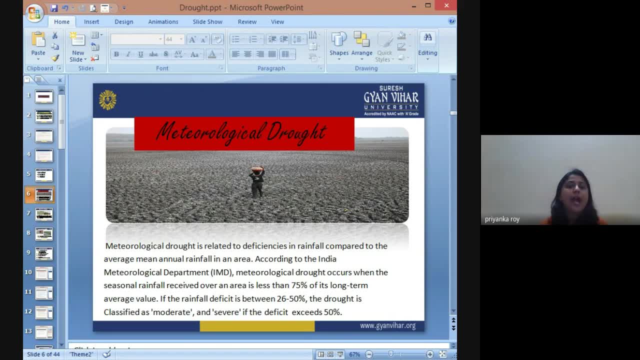 So suppose in this region, in Jaipur, if we have a Rainfall average of about 100, 150 to 200 millimeter annually, So if there is a shortage of rainfall in this year it only falls the rainfall. this year only happens about 100 millimeter. So there is a shortage of water, So it is. 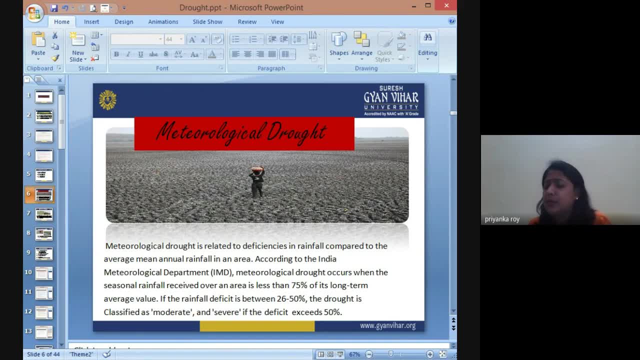 How much It is almost about. you know, 50 to 60, sorry, 75 to 70 to 60 percent less of water, which is supposed to be, So it will have a you know, a significant amount of you know affecting to the agriculture sectors. 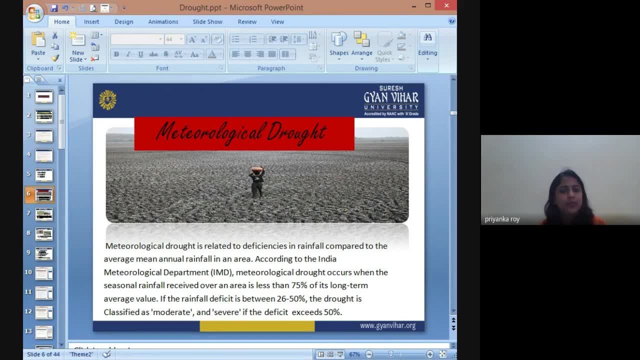 So, according to India, to the Indian metrological department, metrological drought occurs when the seasonal rainfall received over an area is less than 75 percent of its long-term average. So there is a long-term average of 30 years which is taken in consideration when we are talking about climate and weather. 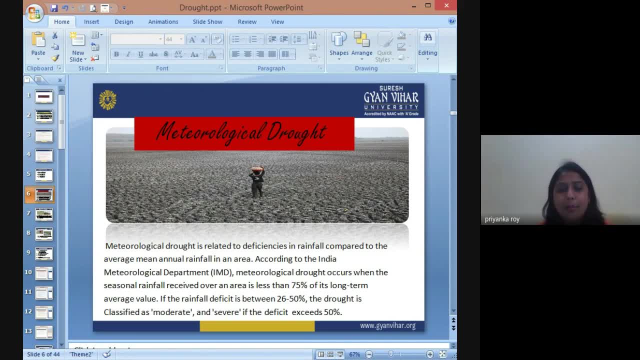 We always take a 30-year span for, you know, any weather pattern to be significantly changing, right? So in over 30 years, when there is a you know, 75 percent less rainfall received in that region, it is pronounced as a drought year. 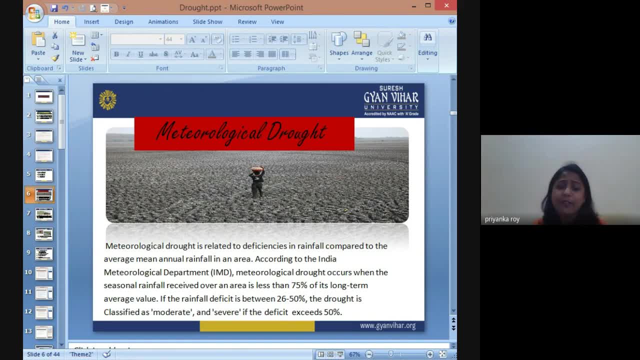 If the rainfall deficit goes beyond 25 to 50 percent. the drought is a moderate. moderate The first one: 75 percent less rainfall. it is just a drought year announced, all right. Well then there is a dry spell, dry year, okay. 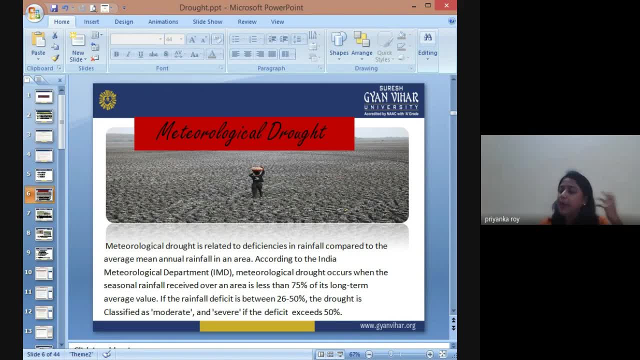 Then the next: if you have 65 to sorry 25,, 26 to 50 percent of the less rainfall and precipitation received in that region, it will be categorized into moderate drought. okay, Now, moderately drought regions. And then, if it is, if the rainfall drops below 20, sorry 50 percent of precise rainfall, then it is called, as you know, a severe drought year. 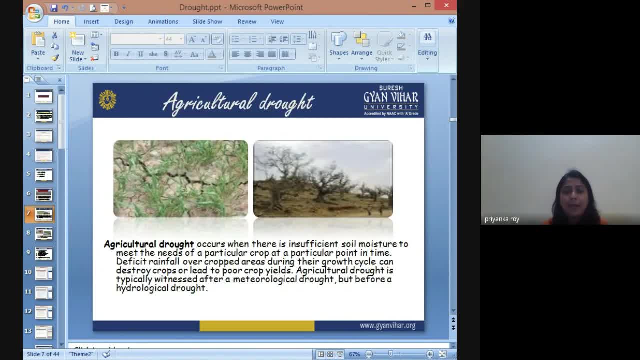 So it will have a very, very severe actions. What will happen here? The agricultural fields will start drying up. So now we are moving towards agricultural drought. Agricultural drought occurs when there is a drought, There is a- you know- insufficient soil moisture to meet the needs of the particular crop at particular point in the time. 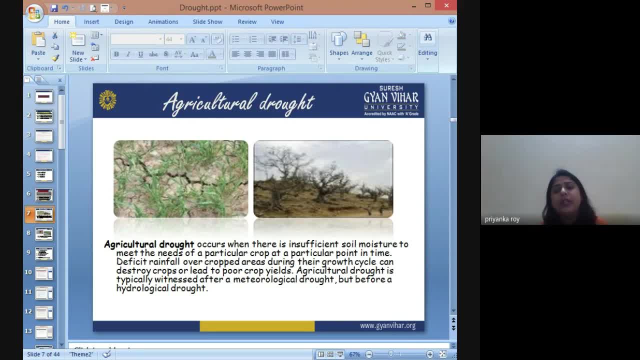 And deficient rainfall over, you know, cropped area during the growing cycle can destroy crops and lead to poor quality of yield. So agricultural drought is typically witnessed after a meteorological drought, But therefore a hydrological drought is also one of the cause of, you know, agricultural drought. 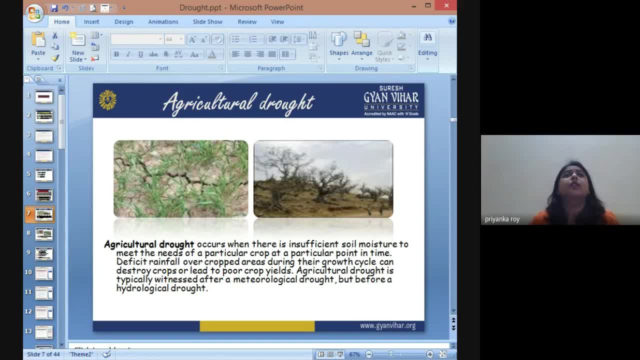 Now, what happens here is, whenever there is a you know less rainfall, which subsequently happening and which will lead up to a dry agricultural land where you know soil will lose out its moisture, the water body will not have water in it. 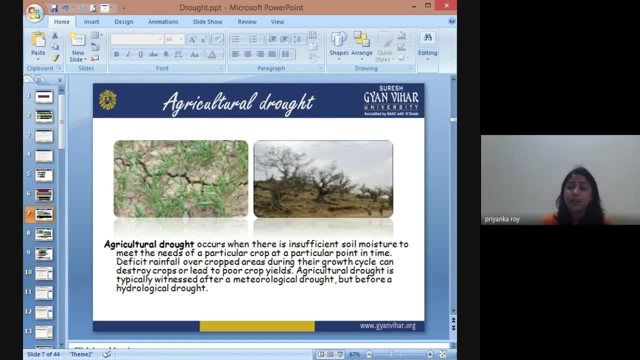 And the irrigation, during the- you know- sowing season or the growing season, of the crops, which will affect the- you know the crop yield, And affecting the crop yield will result in the shortage of food materials, resulting in drought, agriculture drought. 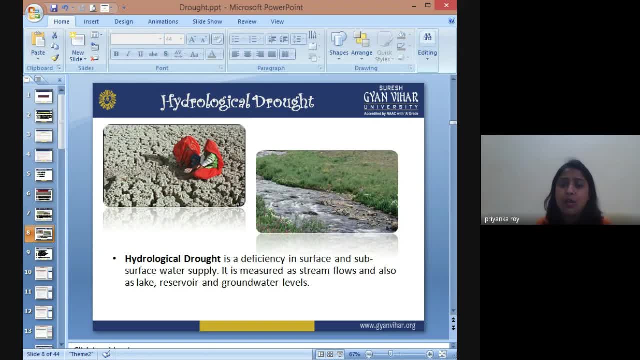 Because there will be a shortage of agricultural product in the market or of a very low quality, which is there. So this is how a you know dry land will look. It will start cracking up because less moisture will start cracking up the soil. 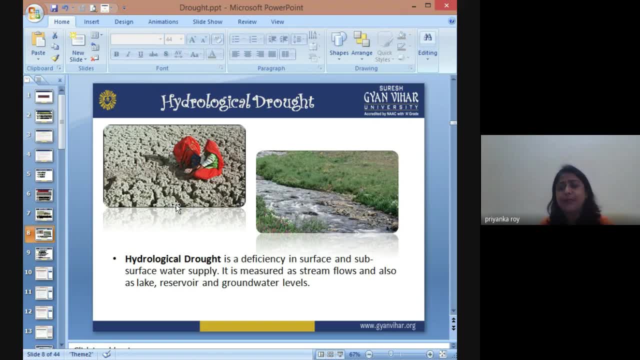 And, furthermore, you know, letting the moisture to escape from the surfaces. Now, how to avoid this? Now, how to avoid this: Hydrological drought is a deficiency in the surface and subsurface water supply. Okay, So when we come to hydrological drought, there is a deficiency of water in the surface and the subsurface supply of the water. 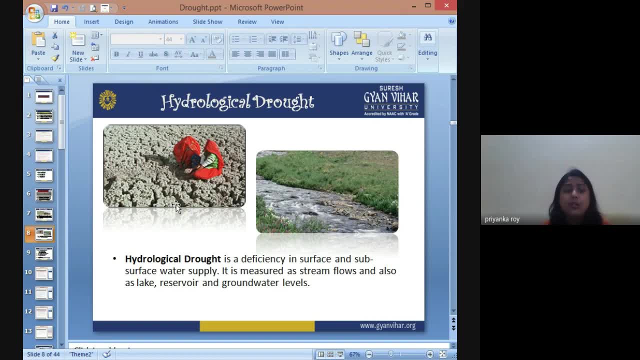 So we can measure it through stream flow and lakes, the amount of water which is contained in the lake reservoir and groundwater level. So by exploring the, So by exploring the areas like groundwater level, by checking the groundwater table, we can identify or we can, you know, at least say that this is going to be a hydrological drought here, as the groundwater has gone down. 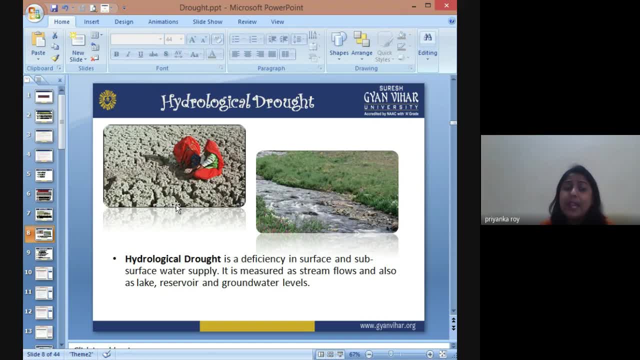 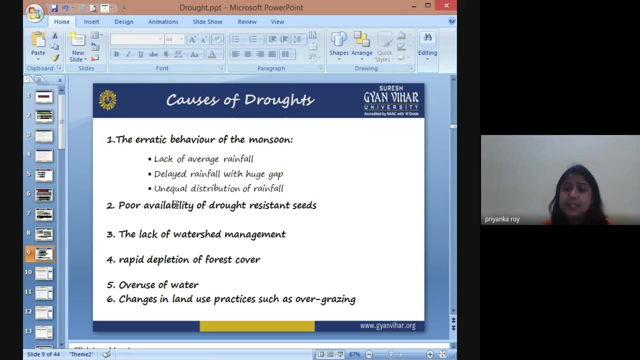 Okay, The surface water has dried up and the lakes and reservoirs does not have enough water to cater for next season, Right? So then it is declared as a drought here where you know. So then it is declared as a drought here where you know agricultural activities will be hindered as it will not be able to irrigate its field. 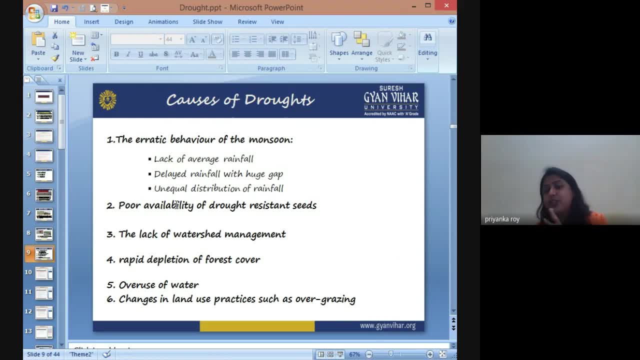 Okay, So now metrological drought and hydrological drought work hand in hand, which affects the, you know the agriculture together. All right, Now, causes of drought. What are the basic factors which causes drought? Okay, So the behavior. 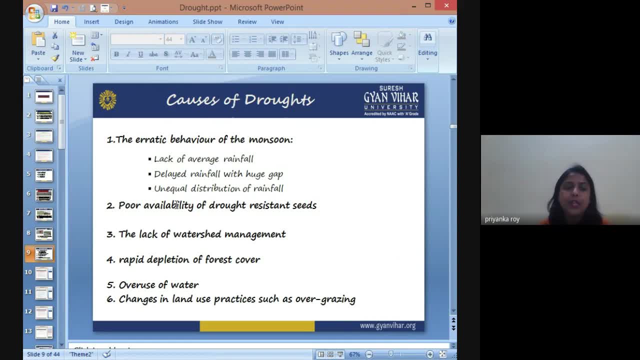 The irregular. You know irregular behavior. You know irregular behavior. You know irregular behavior. The behavior of monsoon, the lack of average rainfall, delayed in rainfall, with, you know, huge gaps of precipitation period, unequal distribution of rainfall, poor availability of drought resistant seeds, lack of watershed management, rapid depletion of forest cover, overuse of water, change in the land use, practices such as overgrazing, and you know. 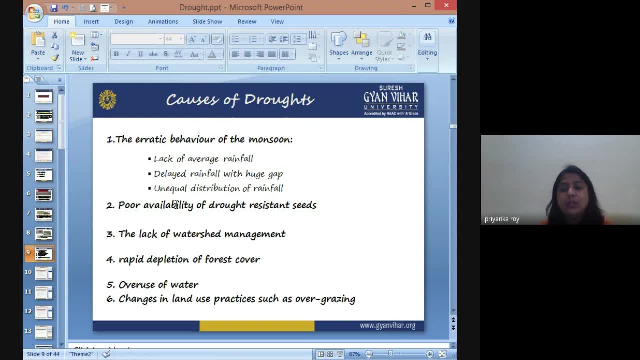 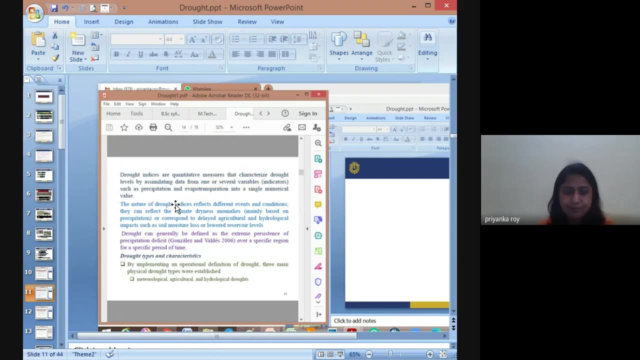 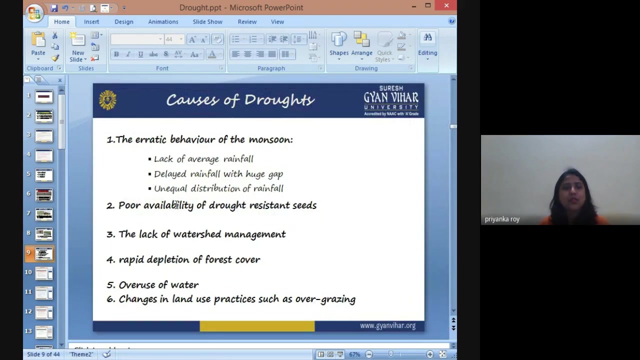 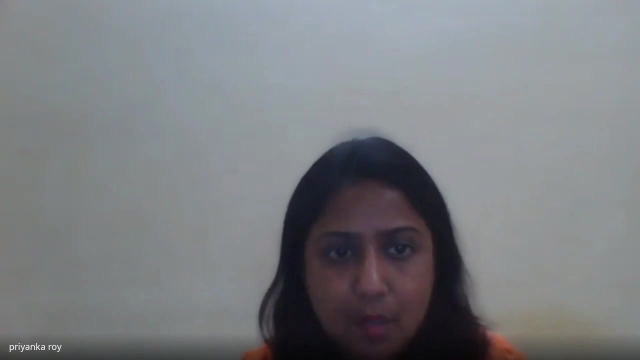 urban expansion, you know, then industrialization- These are some of the causes that will affect the drought here. Okay, Now, Now let's come here. Okay, So what happens here It The erratic, The erratic behavior of any rainfall, suppose in monsoon. monsoon doesn't come properly in time and this undelayed onset of monsoon will delay the- you know, sowing season, right. 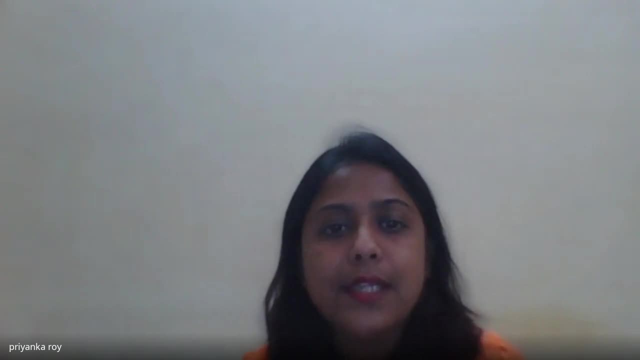 So, as the sowing season is delayed, what will happen is the crops will obviously grow in a delayed time. So the season which is going to up come will also affect the quality of the agriculture products which is going to be out in the market. 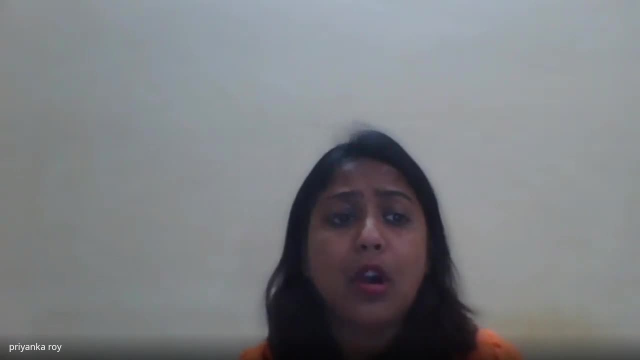 Okay. Similarly, when you, you know, talk about what you called delay and unequal distribution of rainfall, what happens is there are some places on the you know, on your locality, where you will not see any rainfall, not receive rainfall, or uh. you must have seen that during rainy season, one area of your society is 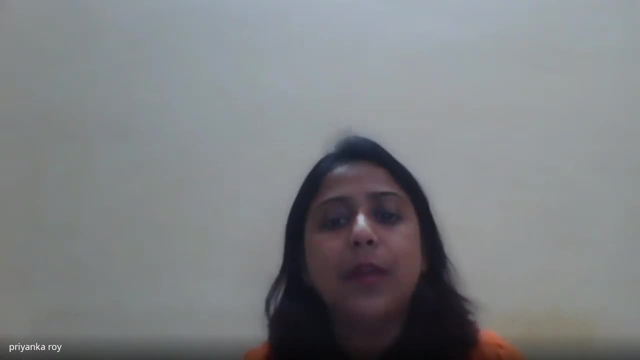 or your city is receiving rainfall. the other part of the city is not receiving much of a precipitation. maybe it is light showers and it stopped. and you talk to your friend- oh, it rained very nicely here. and the other friend will rise to you said no, no, it is not. uh, you know. 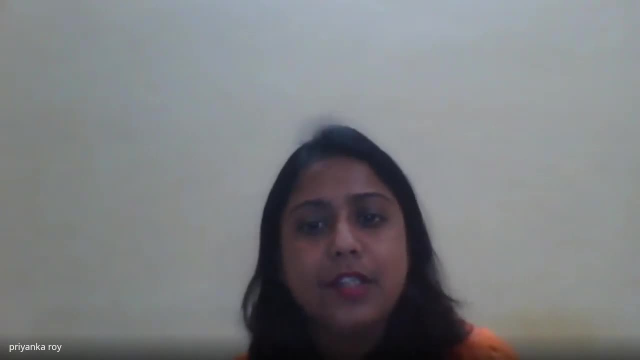 raining here at all, it is just a drizzle. so that is the showing the disparities of various- uh you know- precipitation pattern in the country. so this dissimilar, you know unequal, distribution of rainfall will result in, you know, into dry spells of the agricultural field. similarly, it will also 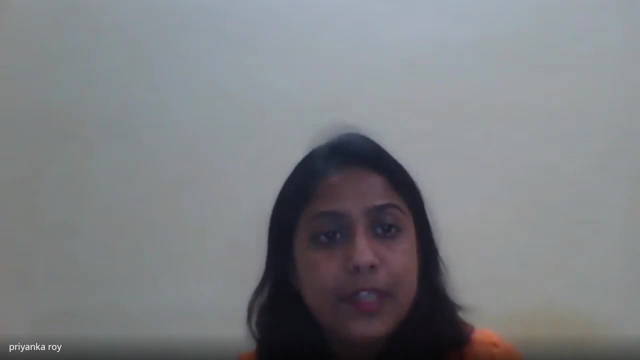 uh, you know, affect the ground water table. if there is a delayed rainfall or less rainfall in that region, it will affect the groundwater table. how it will affect the groundwater table, it will, uh, you know. uh, the water which is, you know, groundwater is continuously, because in modern times we are 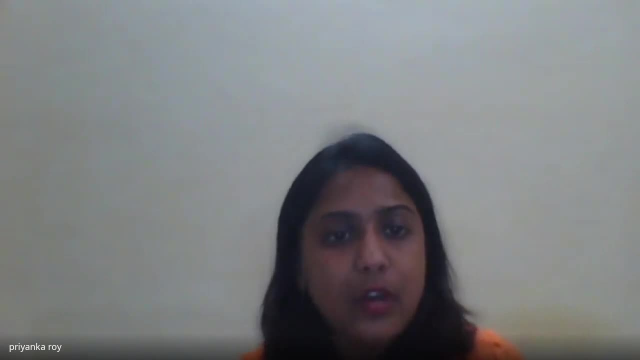 extracting water from the ground. we are exploring groundwater and, with the, for you know, population expansion and other human activities, which is happening to extract water from the ground is, you know, reducing the groundwater table, which is again affecting the agricultural sectors and other domestic purposes, right? so hence, uh, you know, unequal. 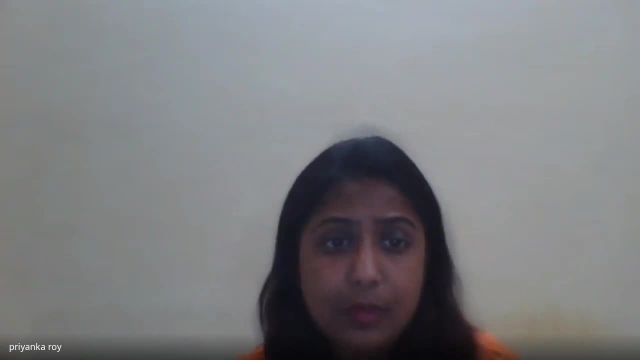 distribution. rainfall will result into depletion of groundwater table. then we have a poor quality of drought resistant seeds. suppose you are growing a agriculture product which is, you know, uh, not drought resistant, okay, which needs a lot of water. let's say a lot of water. let's say a lot of water. 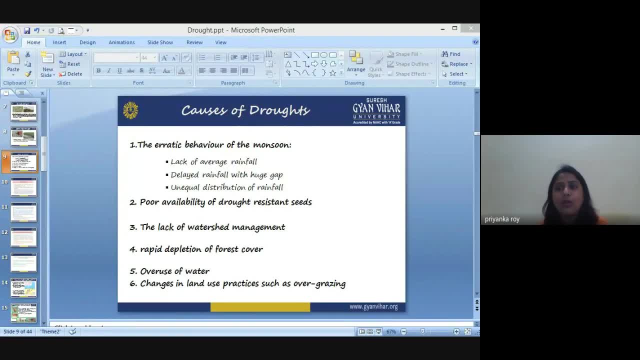 if you grow sugarcane in a desertic region, what will happen? uh, you know, you know it will. sugarcane are known to be a cash crop which yields a lot of money. but uh, has a lot of return, but it will affect the water consumption in that region. so if you saw, 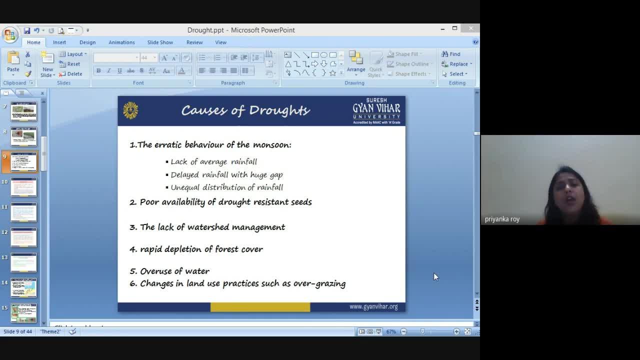 uh sugarcane in a dry area. it will take, it will require more water and if you are not able to give more proper water for irrigation to sugarcane, it will yield less. you know the quality of the sugarcane will be less, all right. hence it will affect the quality, the money in terms of return. 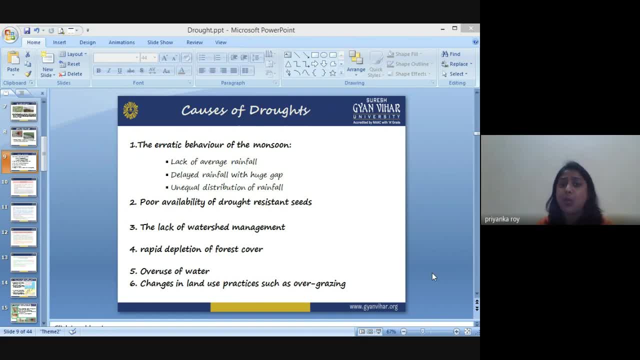 money will be affected. so uh, hence water resistant crops and crops that is according to the region and the weather and the climatic conditions, has to be sown in that area. so poor availability of drought resistant seeds and of the crops and the poor management of uh agricultural pattern will. 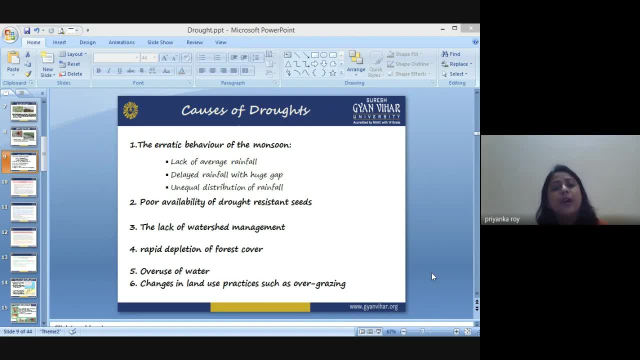 also affect drought. all right, then we have a lack of watershed management. so, uh, even if you reach received heavy rainfall and there is a river flowing around, you know, very close to you, but due to the poor watershed management, your area or your- uh, you know- village is not receiving sufficient. 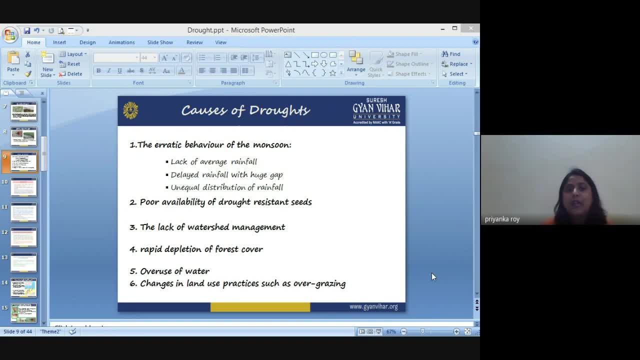 water to irrigate your fields. so that's why you need to grow sugarcane in a dry area for irrigation. So that will again affect that region. in the local matter. it will affect the- you know, irrigation affecting the drought years. So rapid depletion of forest cover is also affecting drought years. as the forest cover is depleted rapidly it is, you know, also taking away a lot of what do you call moisture from the atmosphere. then it is not recharging the natural water cycle. 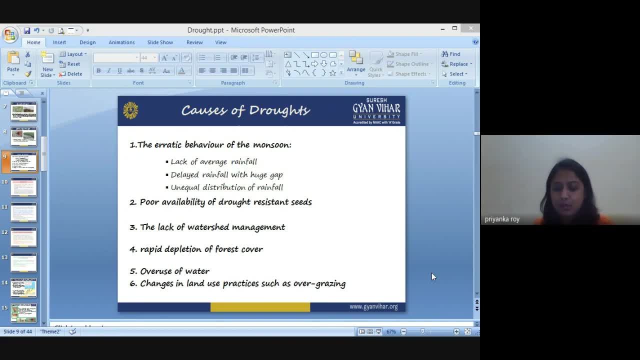 So we know that forest cover, you know, attracts a lot of drought, So moisture on its way right it receives a lot of, you know, rainfall. while it is, you know, there is a dense cover of forest. 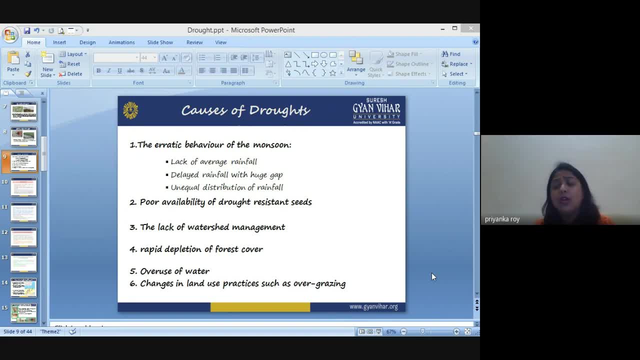 But if you deplete it, if the forest is gone away, the, you know, water cycle is not recharged. Okay, Now, overuse of water. Now, what happens in you know we tend to overuse. We use water, like in domestic purposes, in industrial purposes and in day-to-day life we are using water. 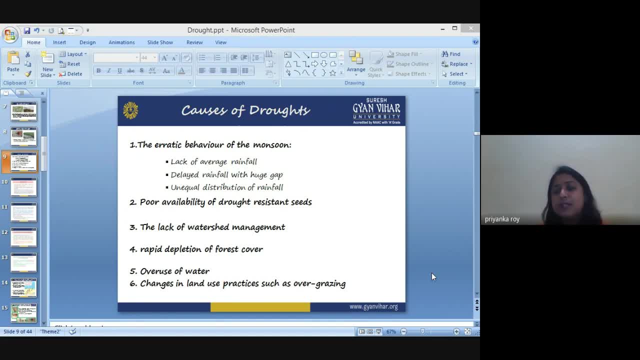 Sometimes we, as in a case of personally using also while you are brushing, there are many people who tend to leave the taps open right. The water keeps on running away. The fresh water is running away, It goes into the sewage, and the sewage water is then needed to be treated and then left into the water body. 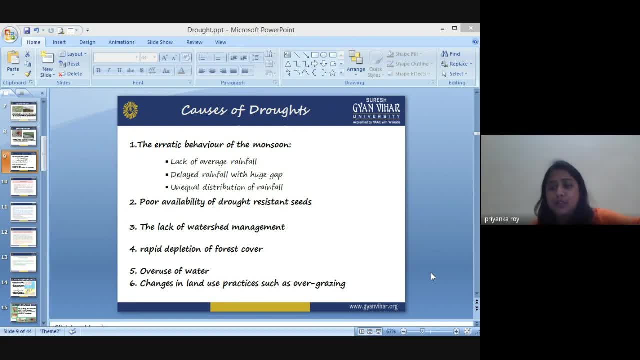 Which again is going to either in some lakes or rivers. right, When it goes into the lakes and rivers it changes the entire scenario, all right. So overusing and misusing of water can also lead to drought years, The change in the land use practices also affecting the drought conditions, 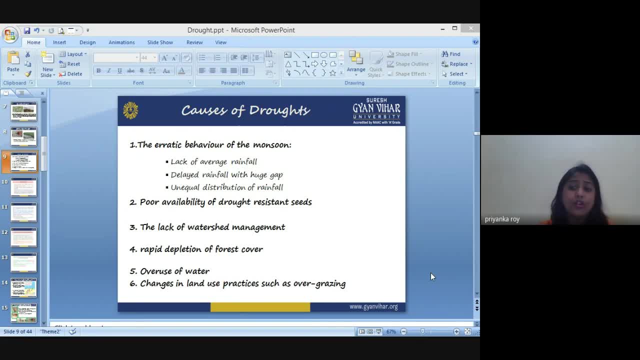 Like we have studied about Chennai flood, where I have taught and told you that these urban area, the Chennai region, has come out to be a big urban region as it has filled up all the- you know small ponds and lakes around. 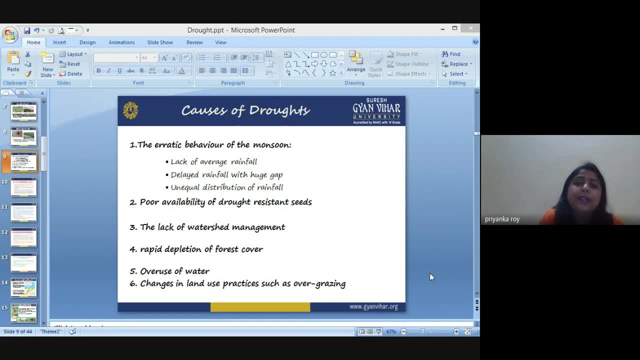 which used to act as a sponge during flood season And they have started, you know, having developmental activities, different infrastructures coming up. Now, along with the, you know, flood years, Chennai also faces shortage of water. Why? Because all the natural, you know, water holes and water tables have been sealed. 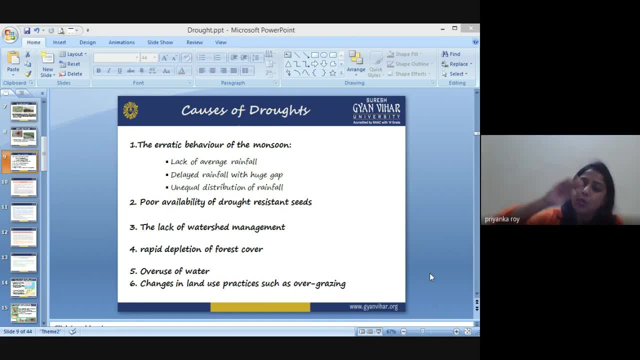 So there The surface water. when the precipitation happens, the water is not circulating under the surface and the groundwater is not able to reach us. Then we are not able to have a proper, you know- water management while the surface runoff is happening, all right. 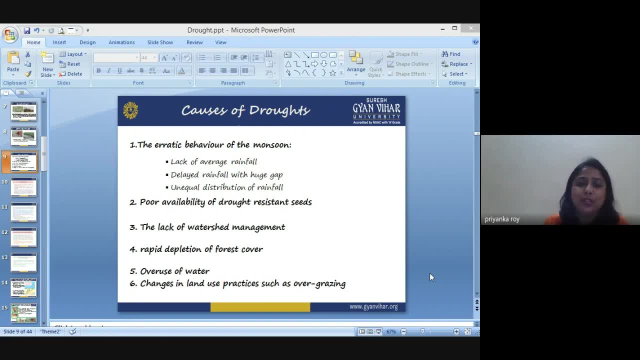 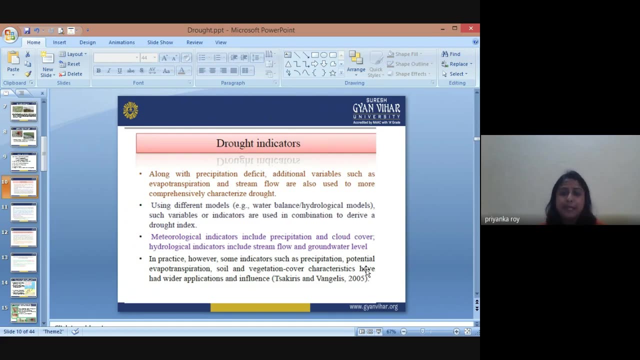 So these are all the causes which will lead up to a drought year. all right, So going to next. Okay, So what are the indicators of drought? Along with the precipitation field depicts, additional variable variables such as, you know, evapotranspiration and stream flow are also used to more comprehensive characteristics of drought. all right, 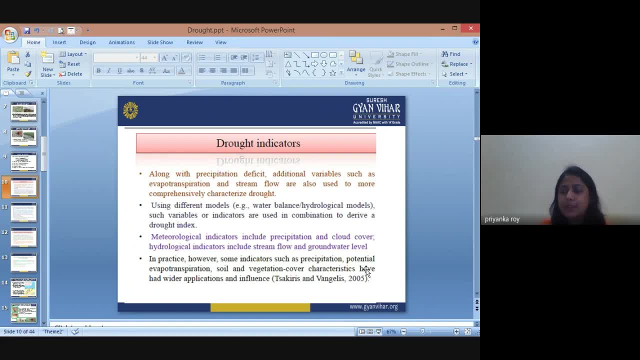 So how do we have a more idea of a comprehensive idea of a drought? here Is that we see that these regions, they have a lot of water streams And every year there's a large amount of- you know- evapotranspiration and evaporation happens. 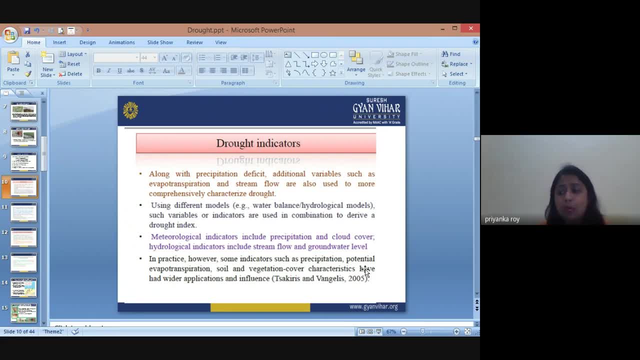 And, as the earth is, you know we are facing a global warming. the evapotranspiration and evaporation process has accelerated. So the use of a balanced model, such as variables and indicators that are used to combine to drive a drought index. 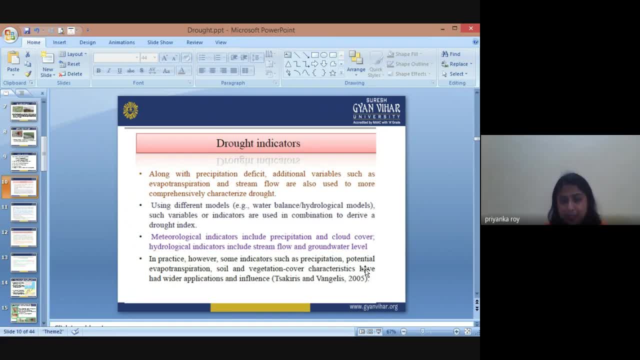 So metrological indicators. So metrological indicators includes precipitation and cloud cover, Hydrological indicators include stream flow and groundwater And in practice, however, some indicators such as precipitation, potential, evapotranspiration, soil and vegetation cover characteristics have had a wide application and influence in the drought indicators. 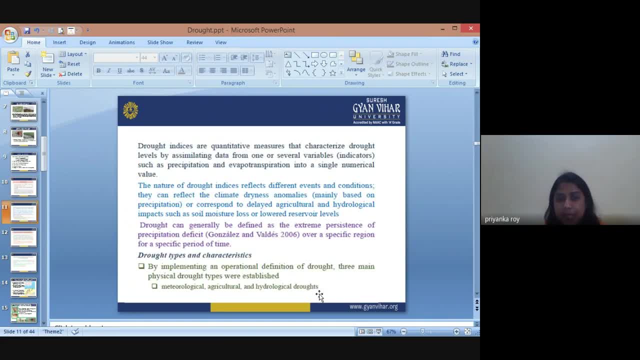 So these are the few indicators that direct us to understand. And then, what has triggered the drought? So, all right. They are also different parameters to measure the droughts also. So drought indices are quantitative measures that characterize drought level by assimilating data from one to several variables, such as precipitation and evapotranspiration, into a single numerical value. 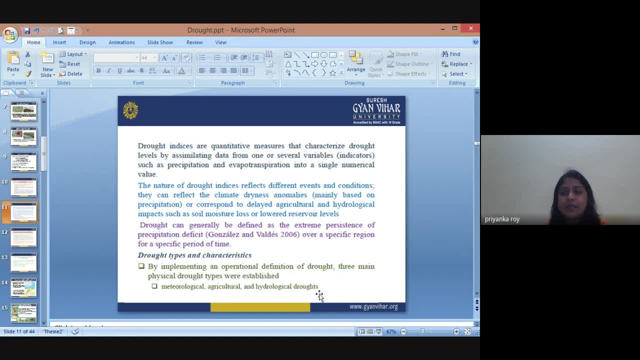 Okay, So precipitation and evapotranspiration. So precipitation and evapotranspiration into a single numerical value. Okay, Now the nature of a drought: indices reflect different events and conditions. They can reflect climatic dryness and anomalies. okay, 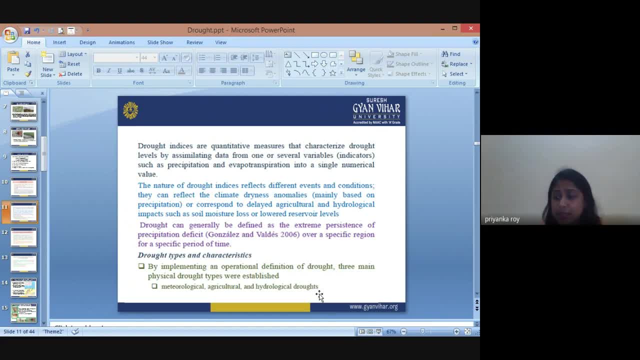 They can reflect climatic dryness and anomalies. all right, and they will. uh, what do you call it? The drought can generally be defined as an extreme presence of, you know, precipitation or deficiency of precipitation. Okay, So what are the various types of drought? we have metrological drought, agricultural drought and hydrological drought. 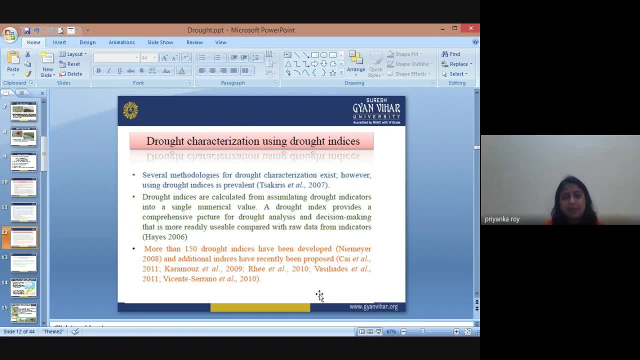 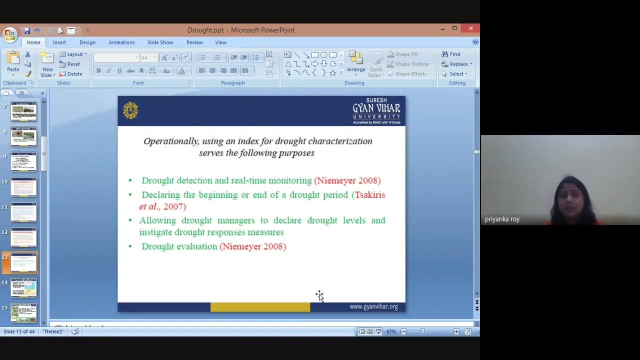 So drought characterized by using drought indices, that is several. you know metrological drought, or you know hydrological drought or agricultural drought have different parameters. OK, now, operationally using the indices for the drought characterization- you know services and follows the purposes of that: drought detection and real time monitoring. 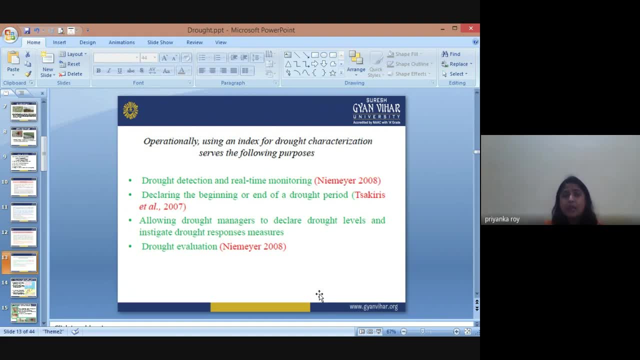 It has been done by Nimir in 2008.. Then Tersky and his authors in 2007, declares that the beginning of the end of the drought period and it has tried to describe how it begins and how it ends, Allowing the drought managers to declare the drought level in the insight. drought response measures. 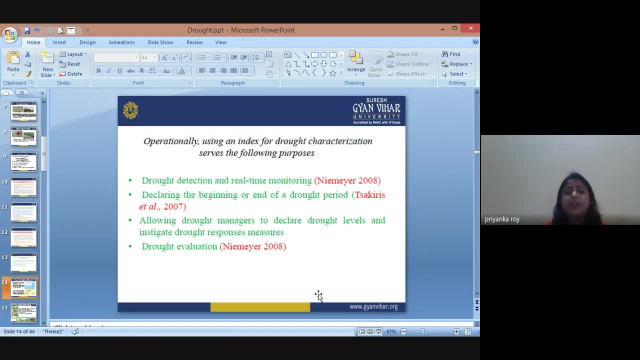 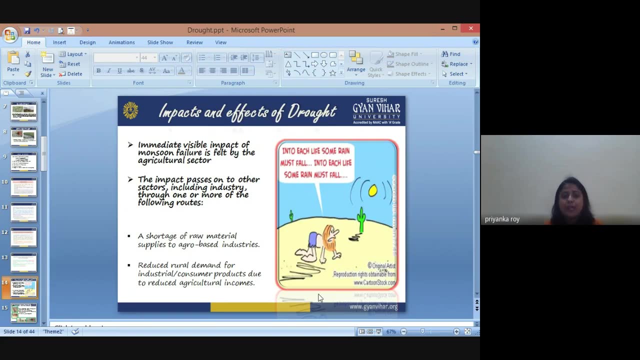 So drought evaluation also was done by Nimir in 2008.. The impact and effect of drought, the immediate visible impact of monsoon failure, is felt by the agriculture sector, So the impact passes on to the other sector, including industries, through one or more mediums like agro, after agriculture. 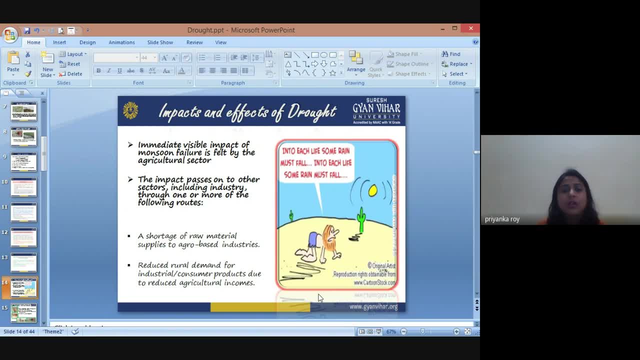 Agro based industries are the areas industries which gets affected by the drought. Then a shortage of raw material and supplies to agro based industries will occur and reducing the rural demand of industrial consumption will increase, accelerating. There is another term which has been newly coined up: is called economic drought, where, you know, due to the lack of economic capability, 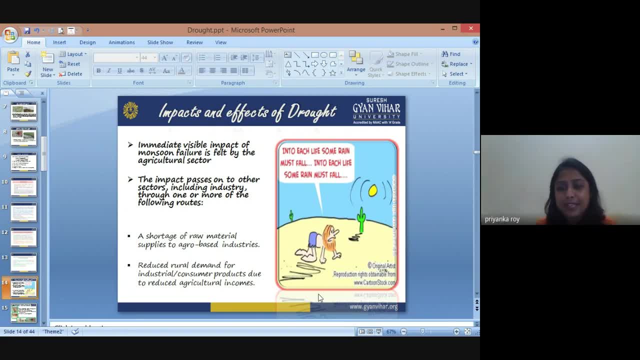 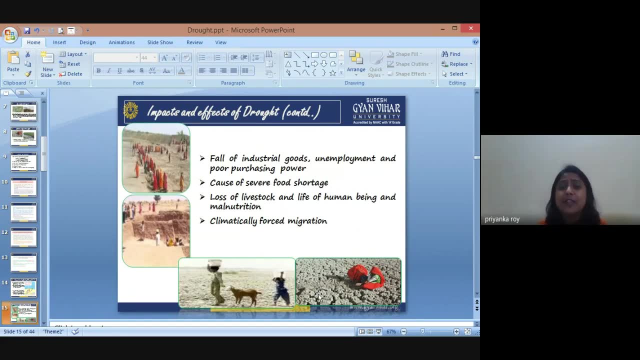 And You have less, you know, agriculture yield, less buying capacity and also economically driven OK. so the impact is it will trigger large scale migration. It will trigger climate- you know climatic force migration, loss of life to livestock, a loss of agricultural product, loss of livelihood and many more. 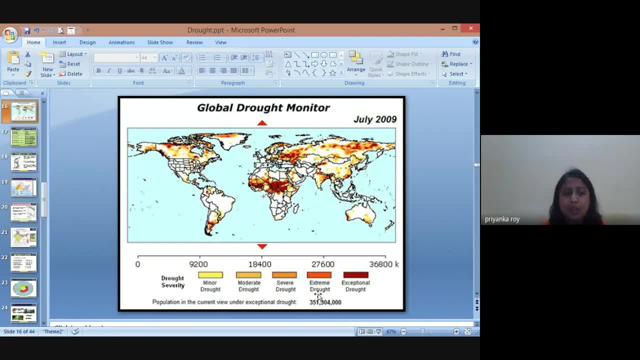 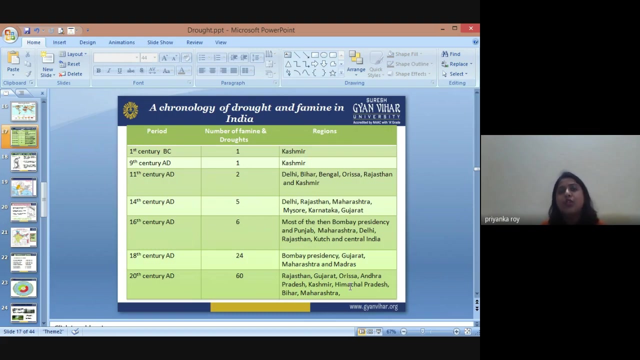 OK, so this is an image which shows the drought monitor, OK, And you see the red lines are the. you know they are very highly drought prone areas. So taking from these region A very highly drought prone regions, OK, Now these are some chronology of droughts and famine which has happened in India, starting from first century BC to the 20th century. 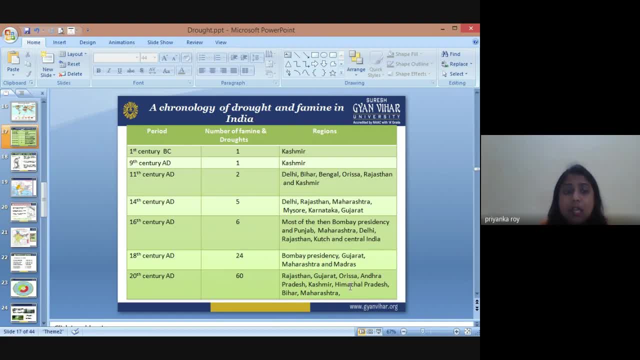 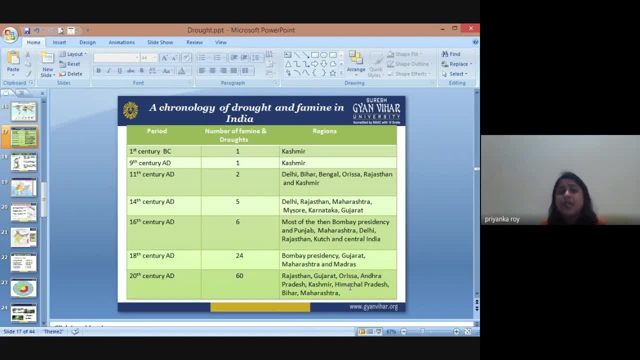 Delhi, Bihar, Bengal, Odisha, Rajasthan and Kashmir. The entire region was affected by drought. Then, 14th century, we had five droughts affecting Delhi, Rajasthan, Maharashtra, Mysore and Karnataka, Gujarat. So now you, as we go, come towards. The 20th century and 21st century, the number of drought prone regions are increasing. So first it started with Kashmir and slowly it started affecting Delhi, Bihar, Bengal, Odisha, Rajasthan and now, after Rajasthan, it has started joining in Gujarat. 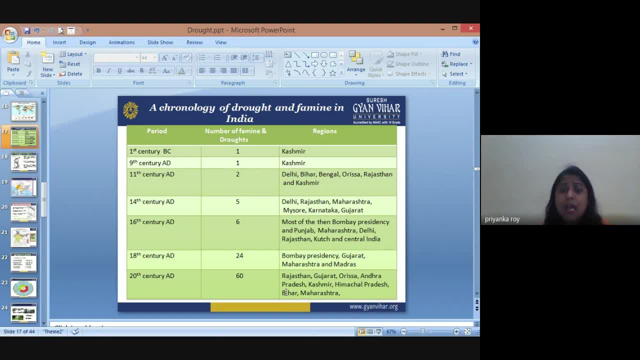 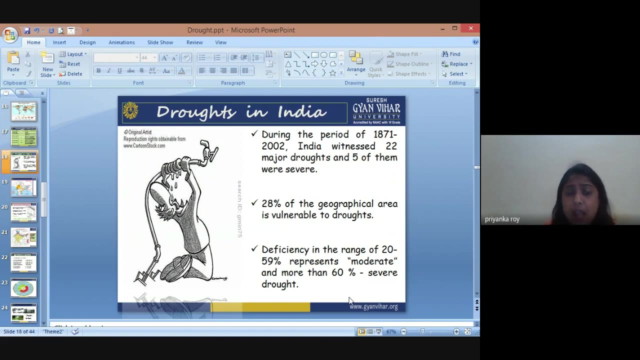 Then you have Himachal Pradesh also being affected by droughts, Bihar, Maharashtra being included in it, and so on. Then slowly, Slowly, the other areas are increasing of the getting drought prone regions. Drought in India have been ever since the timeless modern times. 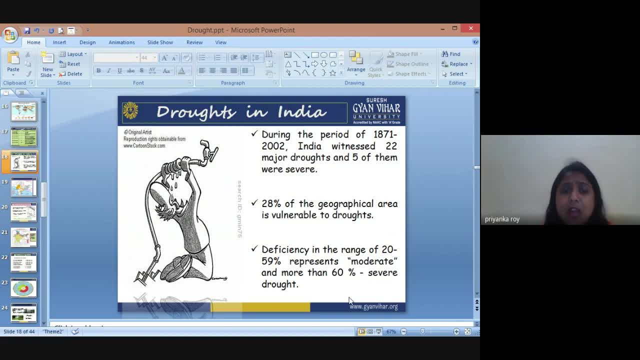 We have seen many droughts and it has triggered severe to severe losses of life and property. OK, the 20 percent of geography, 28 percent of the geographical area, is most vulnerable to the drought, To the efficiency is like the of ranges between 20 to 59 percent is moderate. 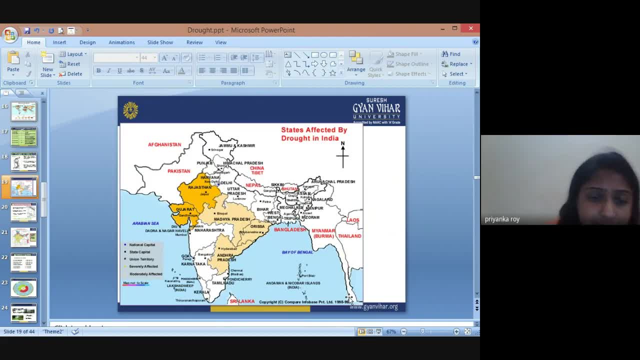 60 percent is a severe job. that is defined by the IMB. India Rajasthan is severely drought prone areas: Gujarat, Maharashtra, parts of Orissa, Andhra Pradesh. Now there is also another state called Telangana And not interior parts of Karnataka.